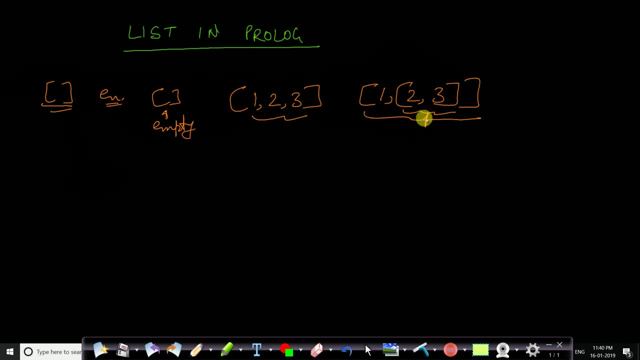 this is the entire list, which is containing another list which is 2 comma 3. okay, so this 2 comma 3 is a single list which is contained within another list. so this is a list of list. okay, so in prologue you have list having two parts. so the prologue list have two parts. one is called head and 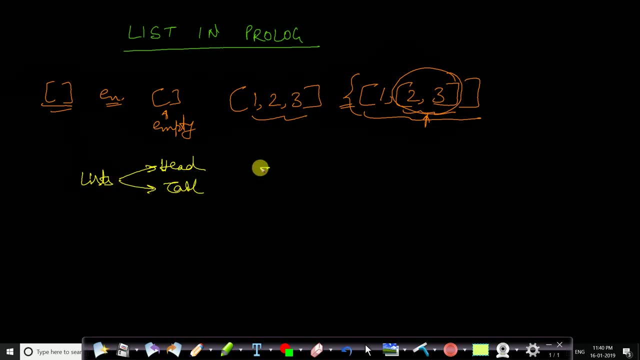 another one is called tell and they are denoted by using this x comma y notation. okay, so this x is the head and y is the tail. so i will just explain you what is head and what is tail. consider this example: 1 comma 2 comma 3. okay, so only the first element of the list is considered. 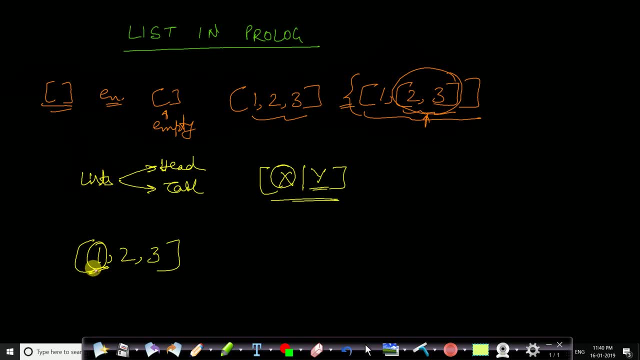 to be head, whatever it is. only the first element is considered as head and the rest all is considered as tail. so here, one is head, okay, and two comma three belongs to the tail, okay, so this is very simple. suppose we take another example like one comma, two comma three, comma four, okay, and this: 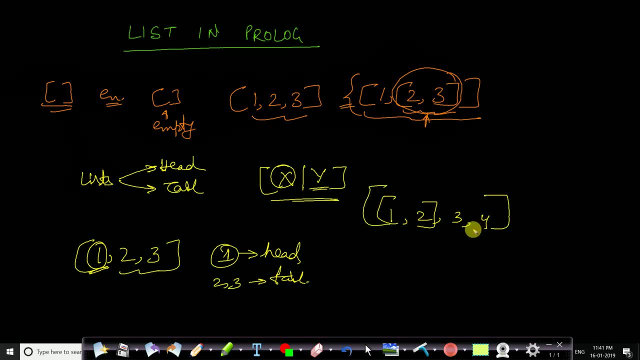 one comma two is a list which is inside another list. so this is a list which is inside the bigger. so this list will be our first element. so here our head will be one comma two. this will be our head because we are only seeing this outer list. okay, whatever is in our first position will be the head. 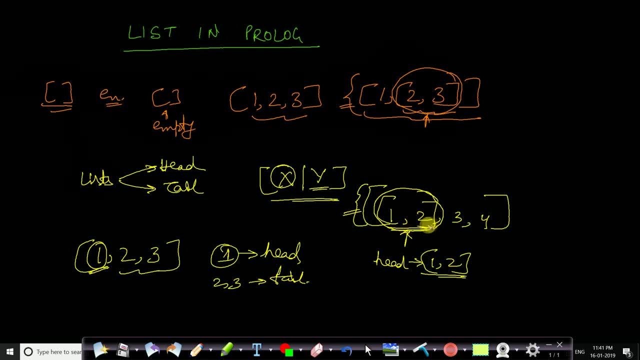 so in the first position you have another list which is containing two elements. so here head will be one comma two, and the rest, part three comma four, will belong to our tail. okay, so this is it about the head and tail. always, the first element is list of the head and the. 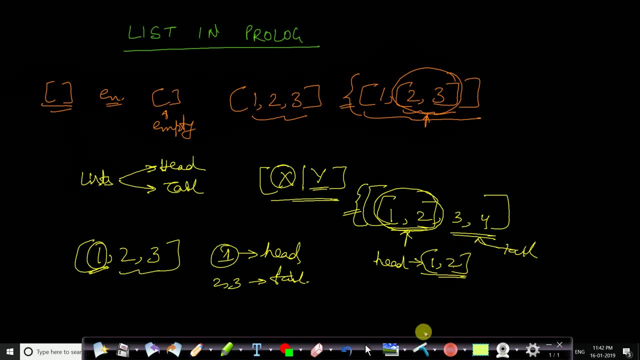 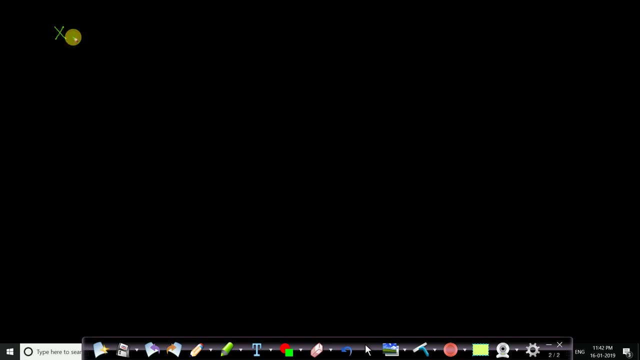 rest all belongs to the tail. you just need to remember this only okay. so let us see some examples in order to understand our concept. suppose i write x comma y comma z. okay, this is the. this will be the third bracket, okay. and suppose i write john, comma likes comma mary. 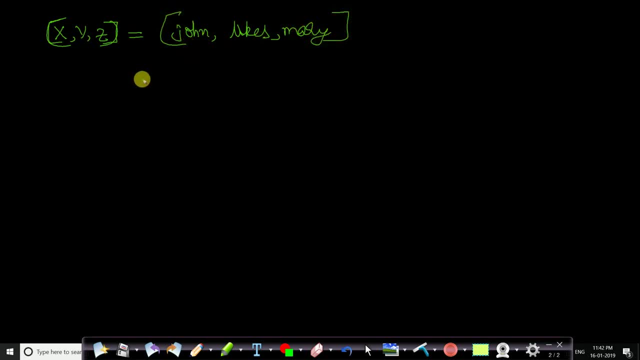 these three are different words, and this is also a list. so by now you must have guessed that here x will be assigned to john- okay. y will be assigned to likes and z will be assigned to marry- okay. so what will be the values here? x will be equal to r- john- okay. y will be equal to likes. 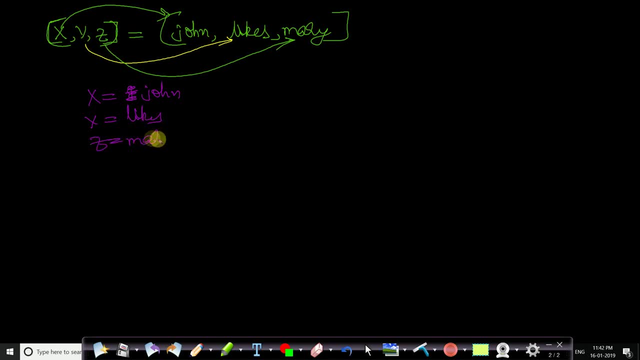 and z will be equal to marry. i will show you by using a code: okay, in sweep prologue. so just first see the theory and understand the concepts. so let us see another example. let us say we write the y: okay, this is a list which is separated by this. okay, so this is denoting that this is our head. 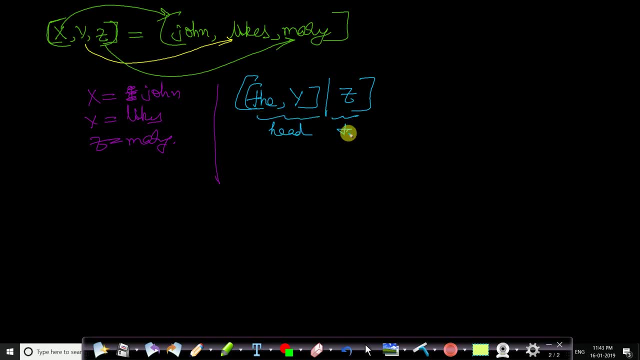 and this is our tail. okay, okay, okay, this is our head and this is our tail. if this is assigned to say some another list where we have x comma, suppose we write mine okay, and again we give is, and then here, then here you can see that this list is having two parts: the bigger list, this one is a. 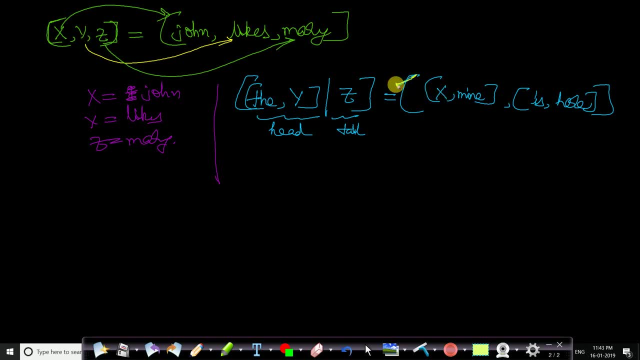 bigger list. okay, this is having two parts. this is the first element and this is the second element, element first and the second element, and you can see that it has been assigned to this one. this is the head and this is the tail. so what will be the head here? head will be equal to the first part. 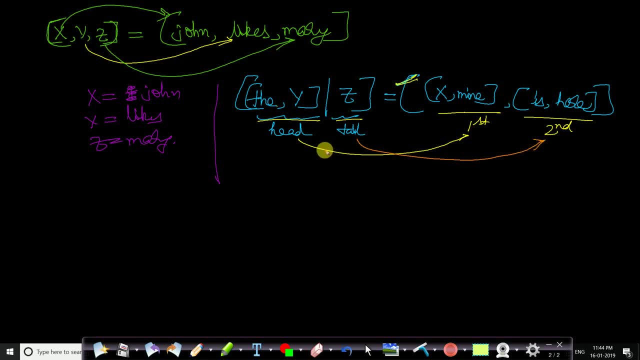 and the tail will be equal to this second part. okay, so you can see that the comma y will be equal to x comma mine. okay, so now you can easily make out that the γ is equal to the value. of a is equals to the valid. you can see that it has been assigned to this. 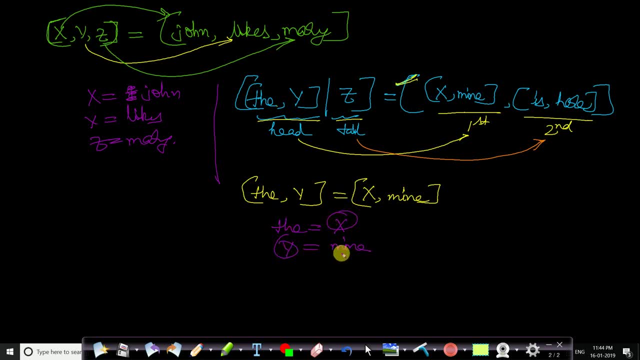 element and in this example you see that this is the value"x'' or the square play, and the cost is $ Shanq pursuing value and the next is the positive. so we'll do the k intense element to the, whether you call, and y will be equal to mine. so the value of x is the value of y is mine. similarly. 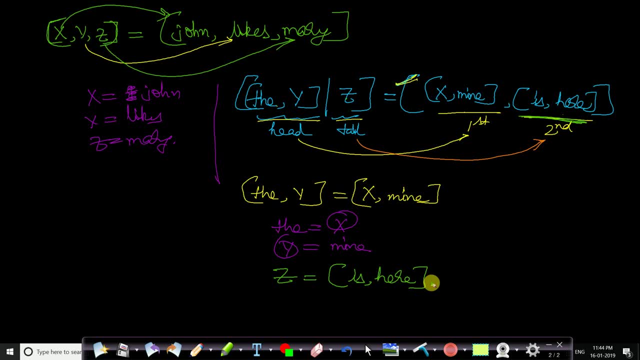 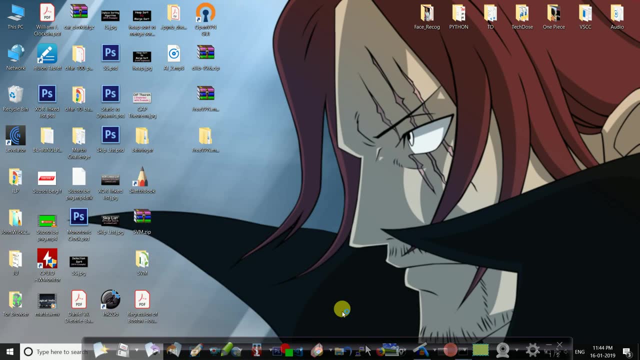 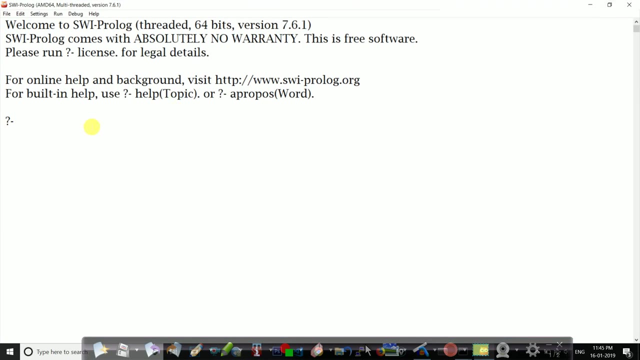 you can see that z will be assigned with this entire second element, so z will be equal to a list. let us see the code in our prologue. okay, so let us open sweep prologue and we will just write some simple code in order to understand. so let us repeat that code which we had seen. 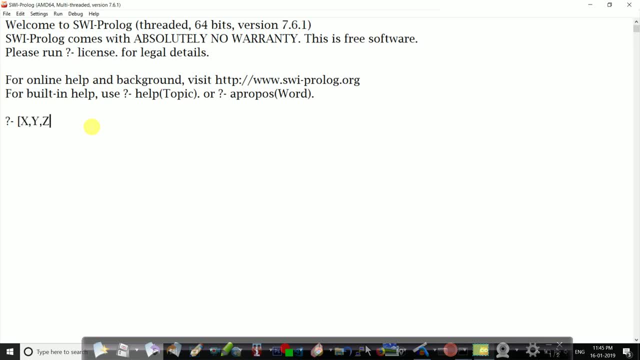 in our explanation, x comma, y, comma, z is equals to, let's say, john, comma likes, comma mary. okay, so, and then give full stop, so you can see that x will be assigned with john, y will be assigned with likes and z will be assigned with mary. let us see the other example which we had done. 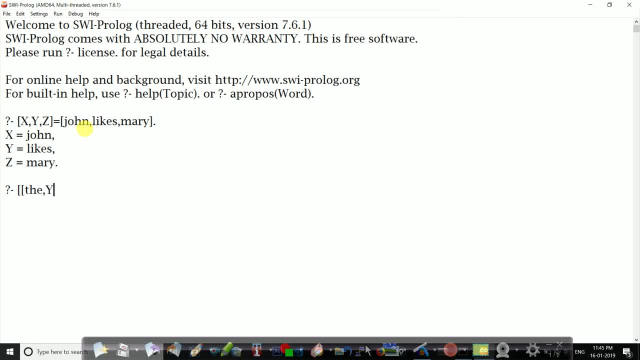 including the list of list, the comma y, and then this will be separated by z. okay, always write the variables using a capital letter. this i have already told you. you can see that this one is a separator here. this one is a separator. let me write it by using: 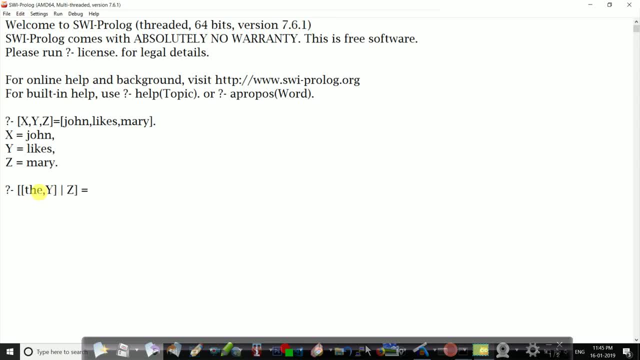 some space. this, the comma y is the head, this z is a tail, and now we will be including another list of list where x is a variable, mine is an atom, and then we will give a comma. then we will include: is here, okay, so you can see that. 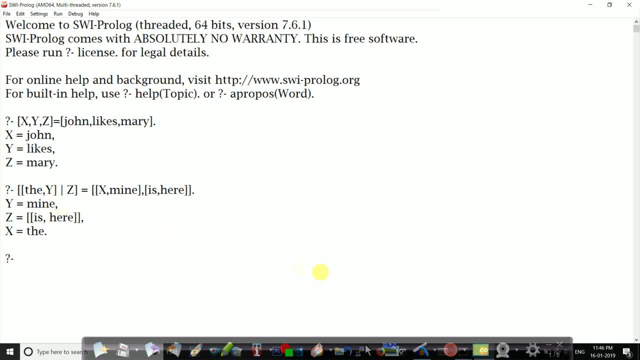 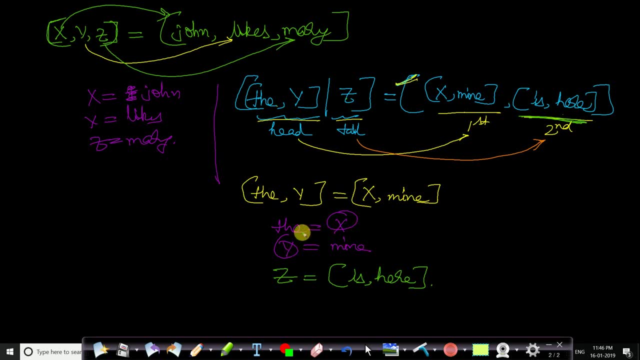 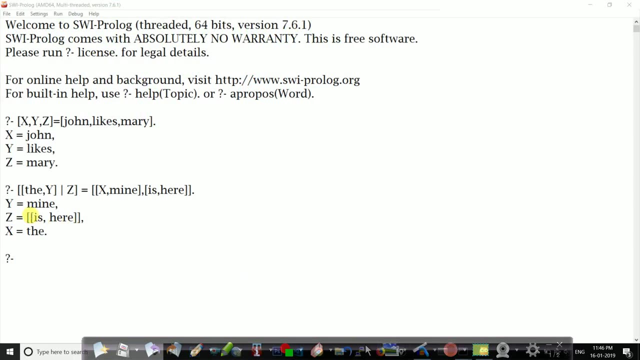 y is assigned with the value mine, as we had seen. okay, as we had seen, you can see that y is assigned a value mine. x is assigned a value. the z is assigned a value, is comma here. okay, so you can see that z is assigned a value, is comma here. x with the and y with mine. so i hope. 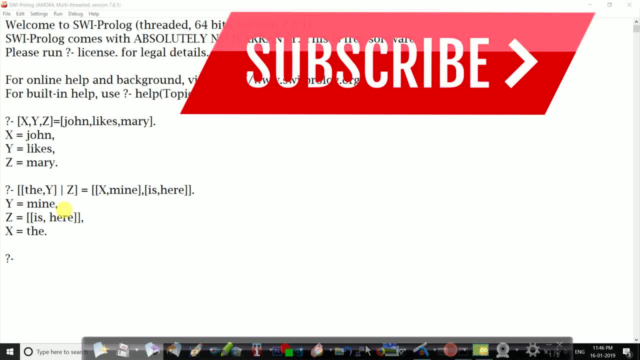 you were able to understand the basics of list. we will see more about list in our upcoming videos, so please subscribe to our channel in order to watch more prologue videos and more programming videos as well. see you in our next video. thank you.